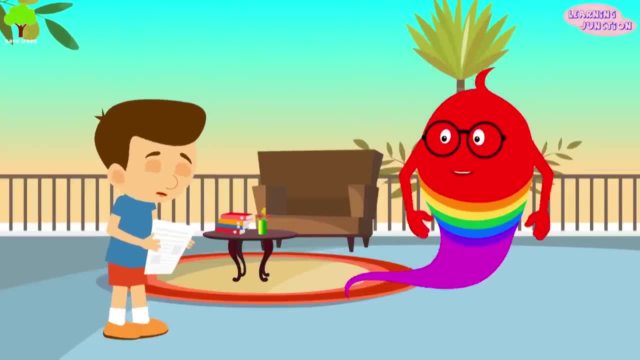 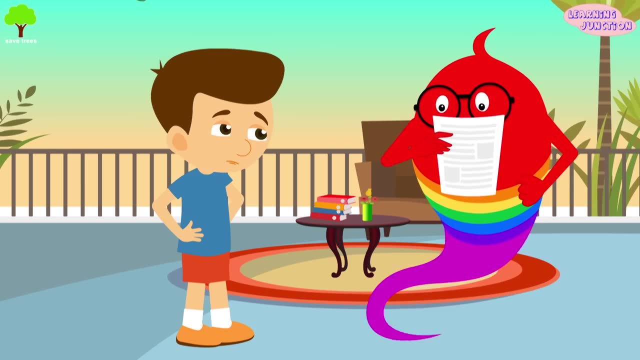 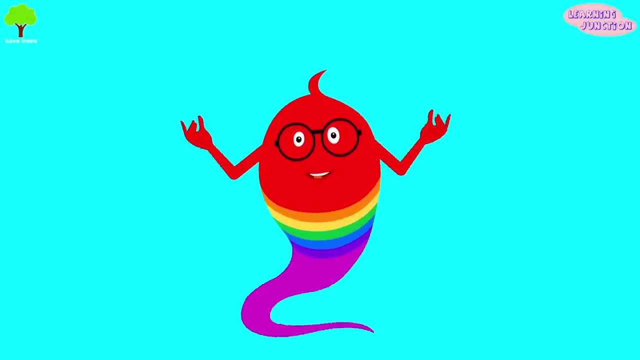 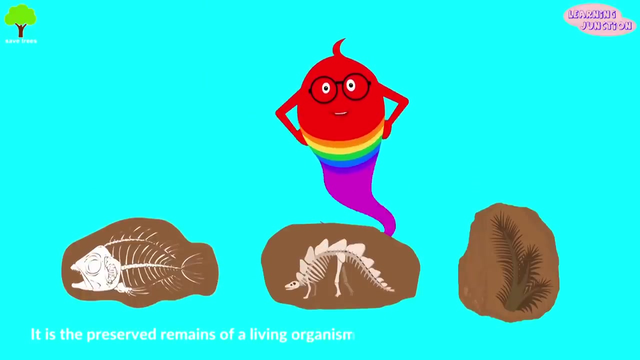 Hey buddy, what's up? Oh, you have an assignment on fossils. Let's learn about fossils today. Fossil is the word we use to describe a wide range of natural artifacts. It is the preserved remains of a living organism, such as a plant, insect or an animal. The word fossil comes from 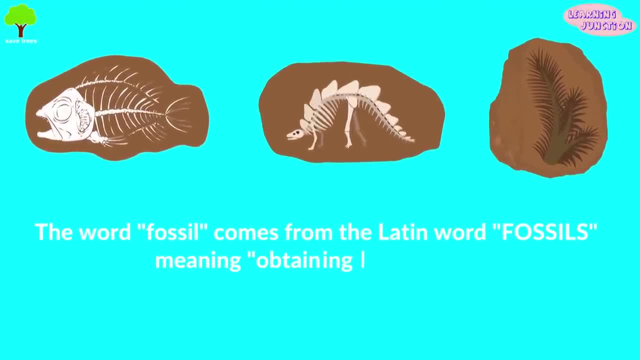 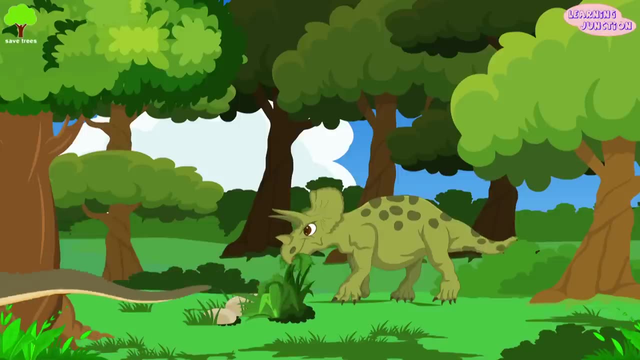 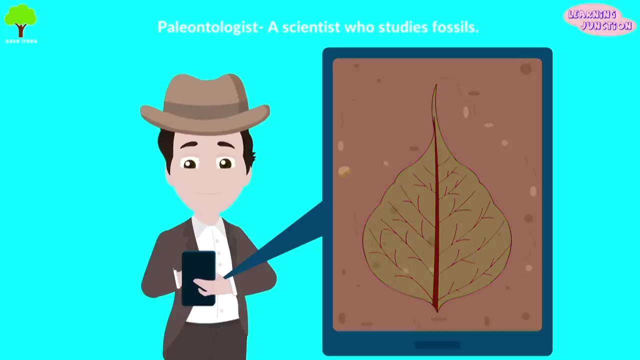 the Latin word fossils, meaning obtaining by digging. Fossils are very important for us if we want to know what happened before us or before our time. The scientists who specialize in studying fossils are called paleontologists. Let's learn about types of fossils: Trace fossils. 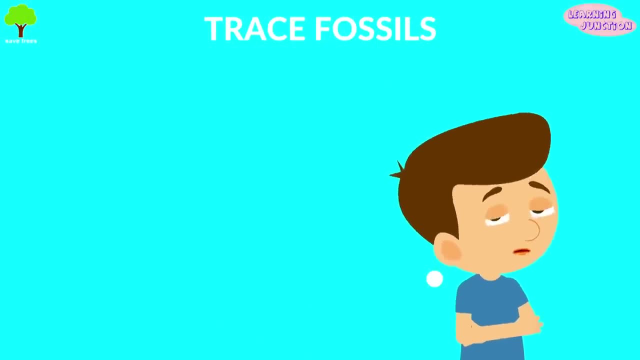 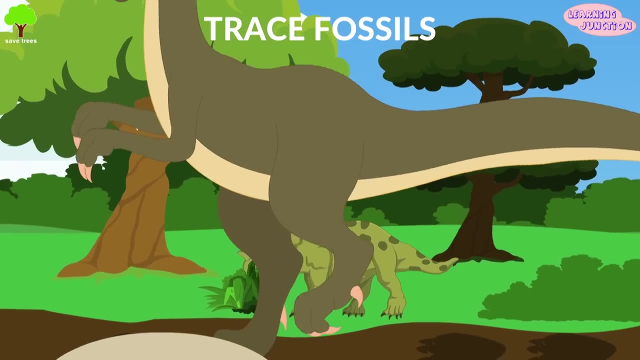 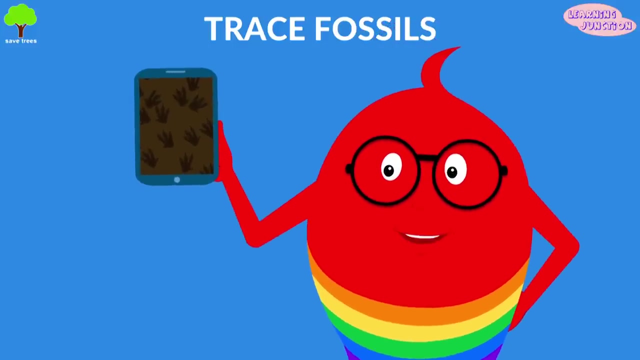 what happens when you step in mud. Millions of years ago, when dinosaurs roamed the earth, they also made large footprints. Fossilized footprints are called trace fossils because they were made by the activity of the dinosaurs. Footprints can tell about the size of the animal. 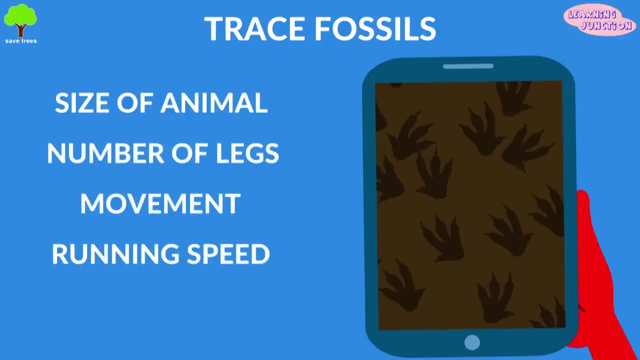 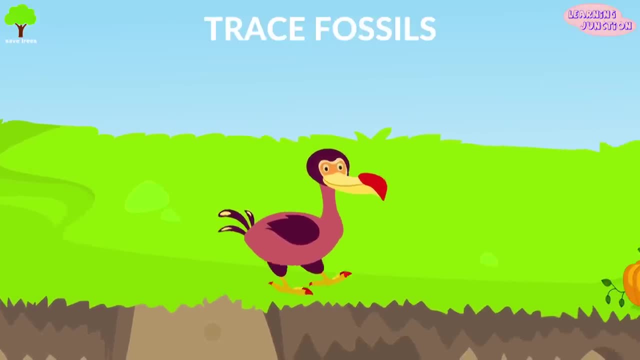 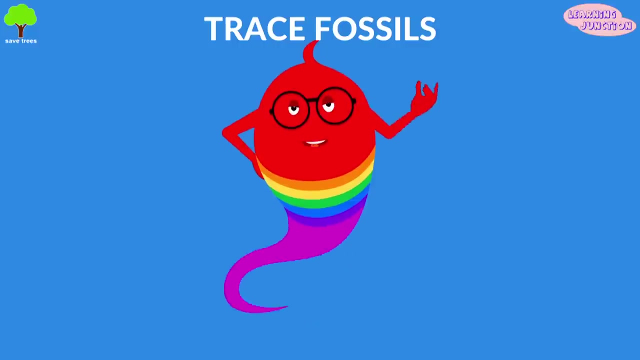 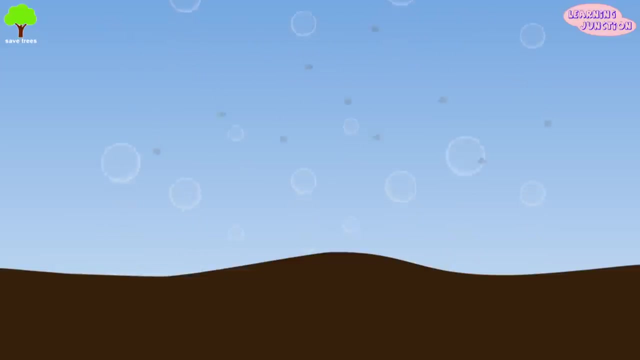 number of legs they had, how they moved and how fast they could run. Ancient fossilized homes of animals: tell us about how and where ancient animals lived. Any fossil that explains the activity of ancient creatures is a trace: fossil Burrows, borings, footprints and root cavities, Mold fossils. Mold fossils are fossils. 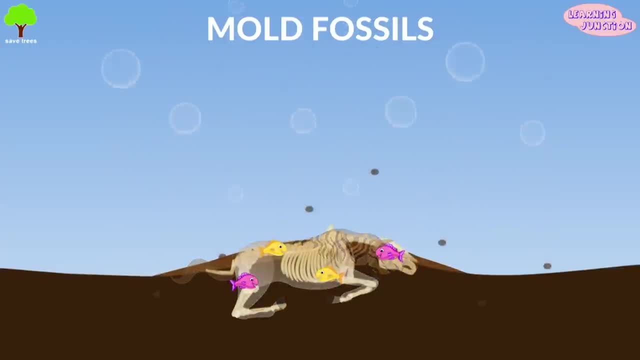 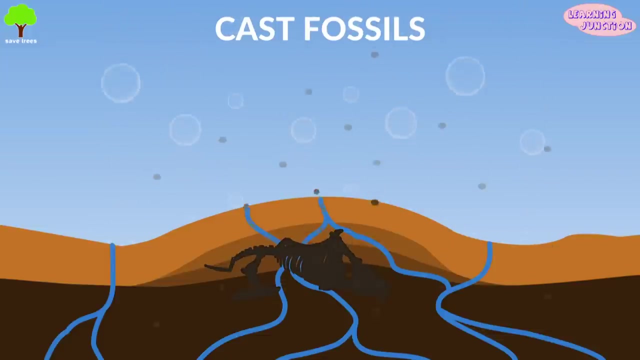 formed when a plant or animal dies and is covered by sediment. Its flesh decays with times and bone deteriorate and it leaves a cavity below the ground surface. Cast fossils: It is formed when the formed mold fossil is filled in by surrounding minerals and sediment. It is a replica of the 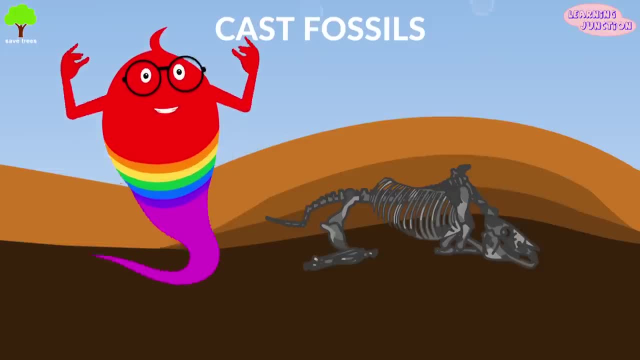 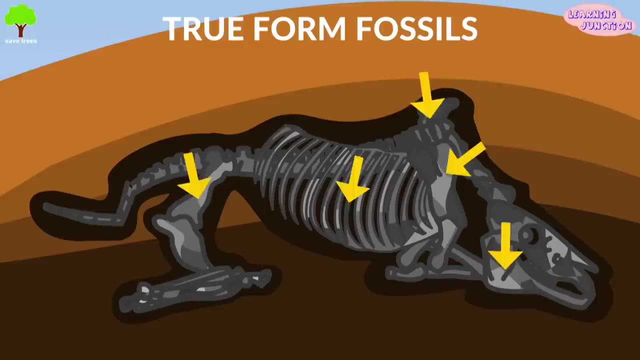 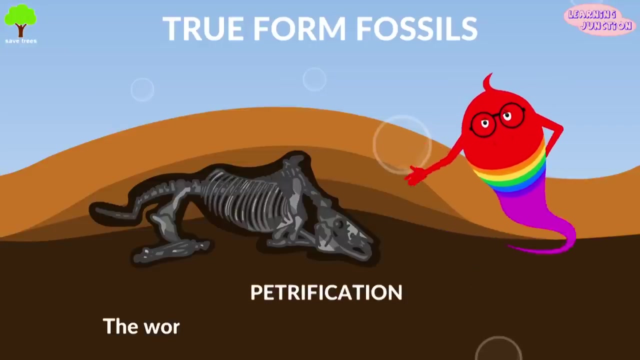 original organism and provides an impression of the original structure. True form fossils: These are large body parts of an organism that has been replaced by minerals. It's created by a process known as petrification. The word petrified means turning into stone. These types of fossils form: